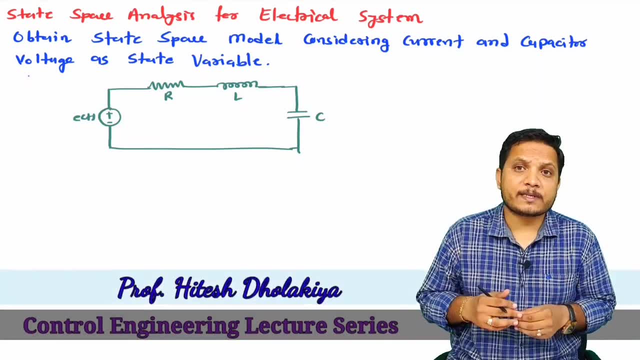 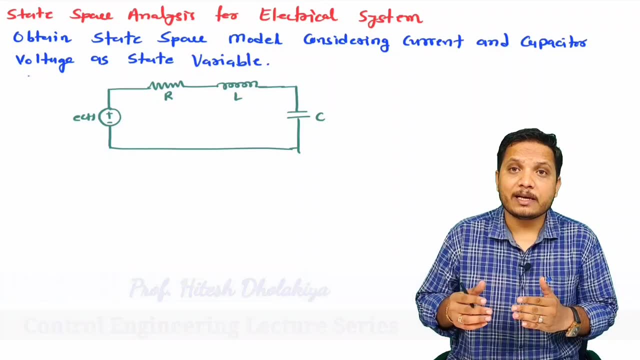 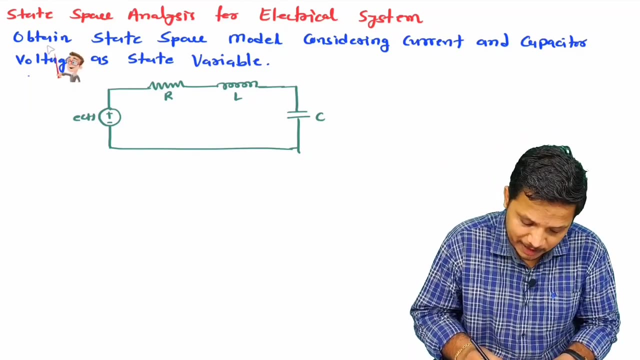 Welcome to control engineering lecture series I. professor Itesh Dholakia is going to explain you very interesting example based on state space analysis, in which I'll explain you state space analysis for electrical system. So let us see the question first. So here you see. 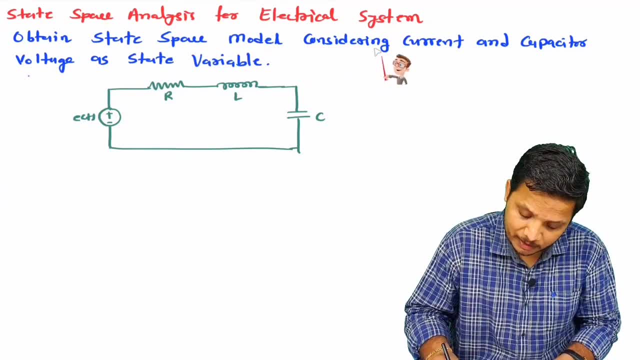 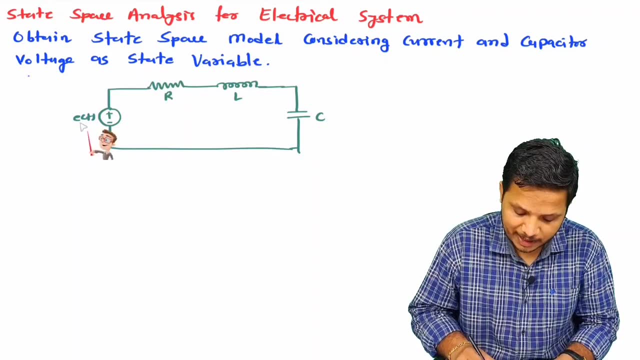 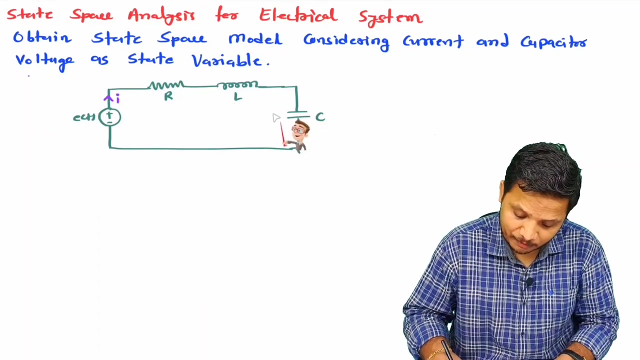 we are delivered to obtain state space model considering current and capacitor voltage as a state variable. and you see here E of T, that is our supply, and RLC circuit is connected. you can observe in that we are delivered to consider current I and capacitor voltage, Vc. 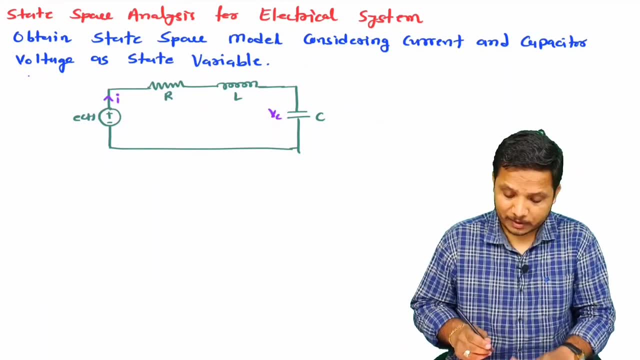 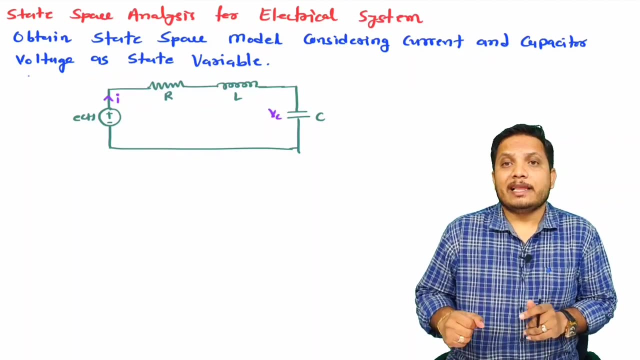 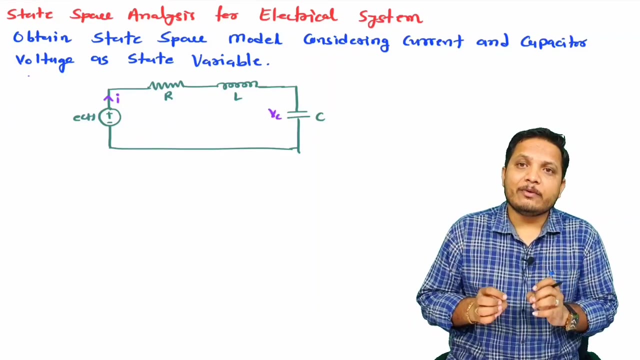 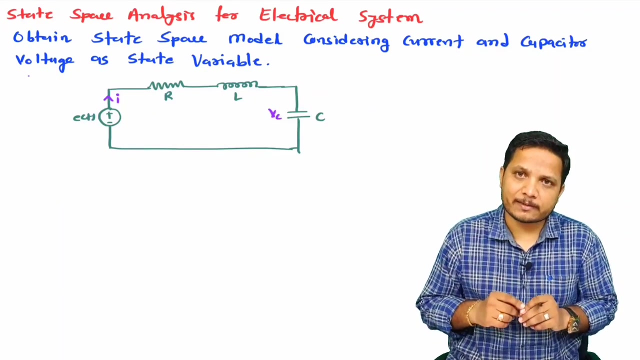 as a state variable. Now, here there are few basics that I would like to discuss first. Whenever you have any electrical network, at that time, first of all, you will have to see how many inductive and capacitive components are there, and based on that we can identify number of state variables. 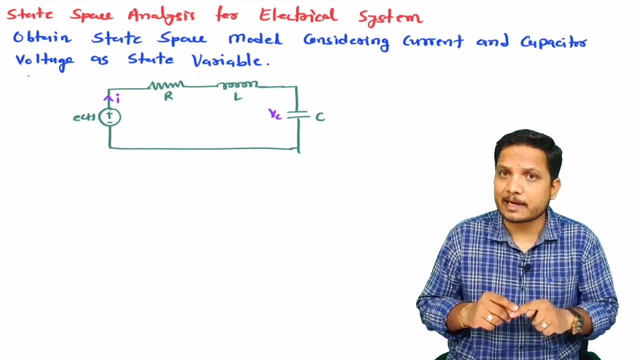 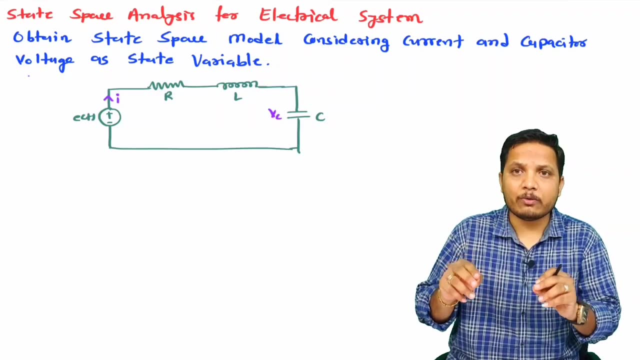 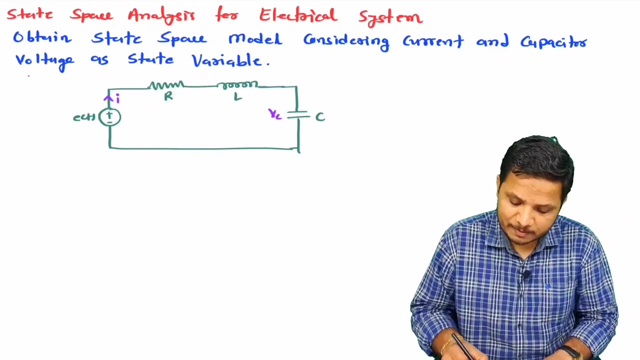 Here, if you observe our circuit, which is RLC circuit, in that inductive and capacitive elements are two. So obviously we will have to have two state variables to have a state space model right. So here state space model will be having two state variables and here 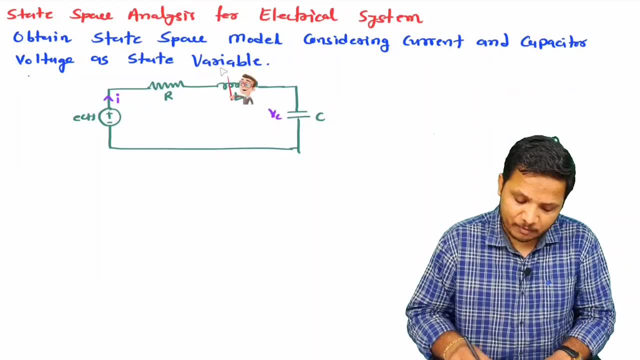 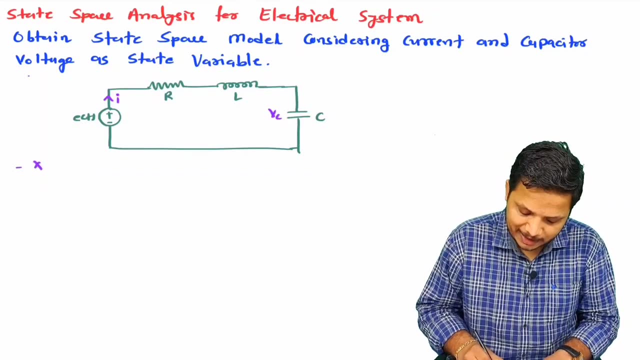 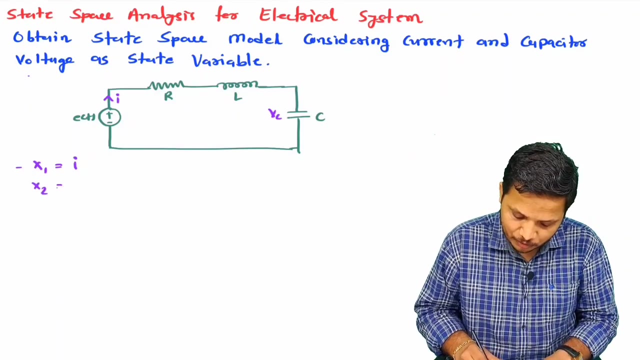 in question itself. it is given current and capacitor voltage that is given as state variable. So let me consider that as a state variable. So let us say X1, that is current I, that is our one state variable, and second is X2, that is capacitor voltage, Vc, that is our state. 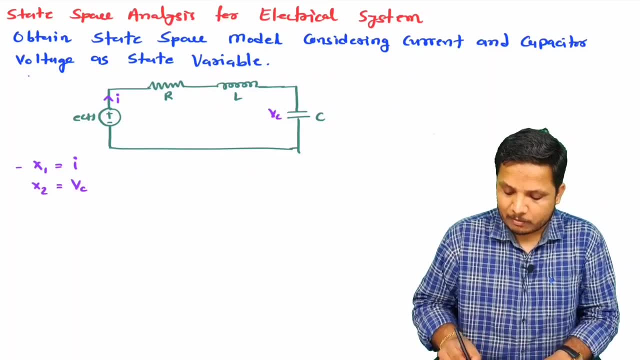 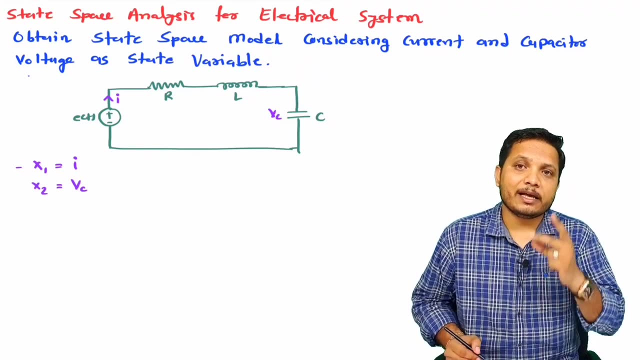 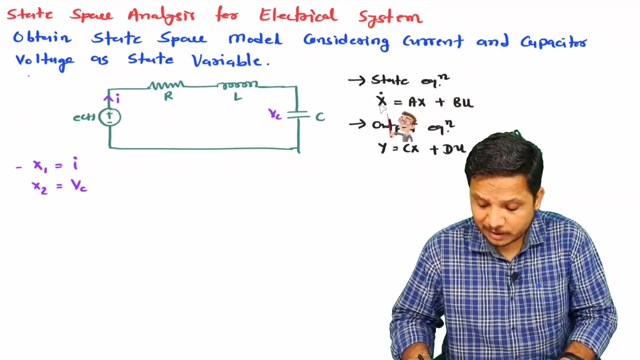 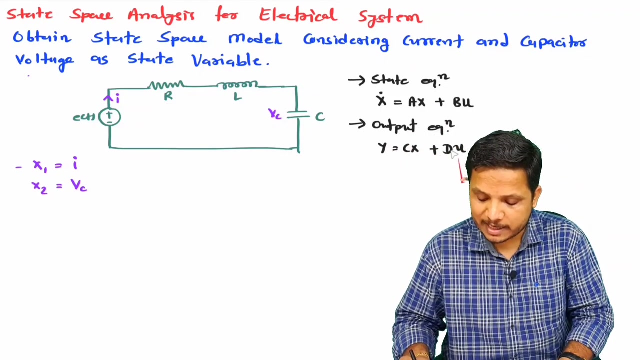 Now, to have state model, we need to have two equations right. One is state equation and second is output equation. and those equations are: state equation that is X bar is equals to AX plus BU, and output equation that is Y is equals to CX plus BU. See in these equations: 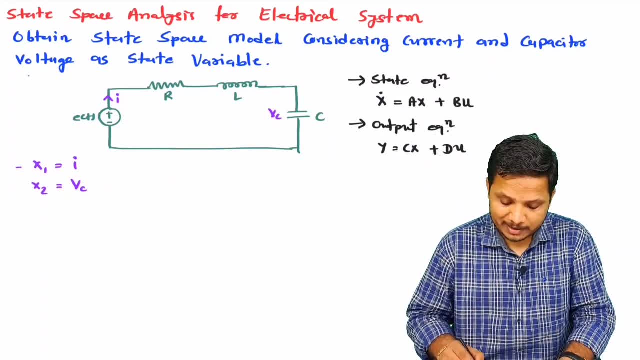 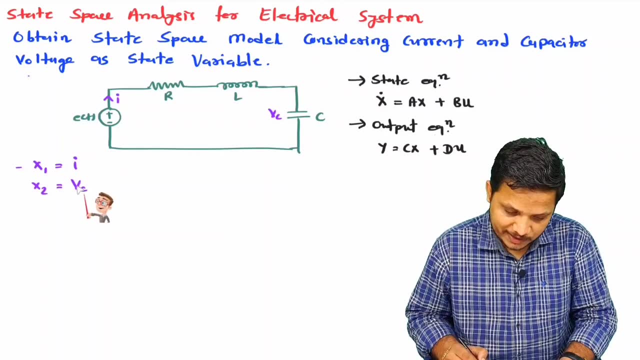 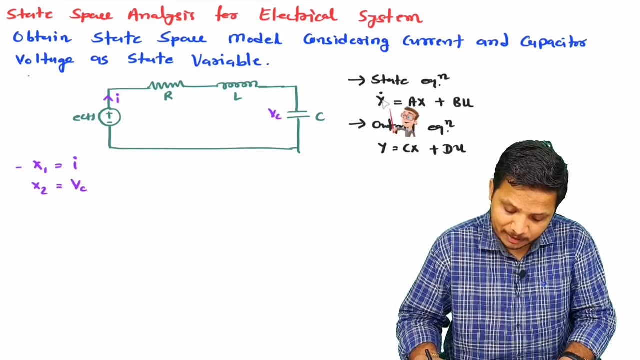 we will have to translate this circuit right By considering X1, that is our current I, and X2, that is voltage Vc. Now, to have X bar equation, we will have to have X1 bar and X2 bar in terms of equation, which is there in terms 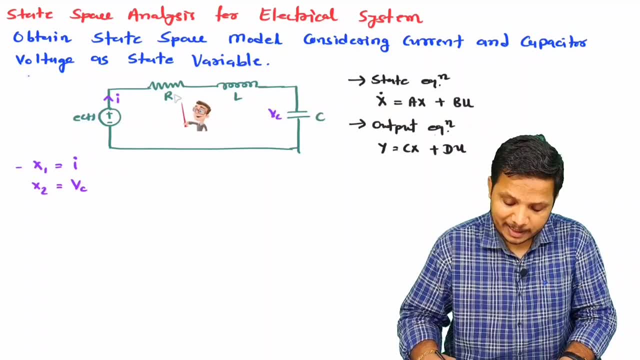 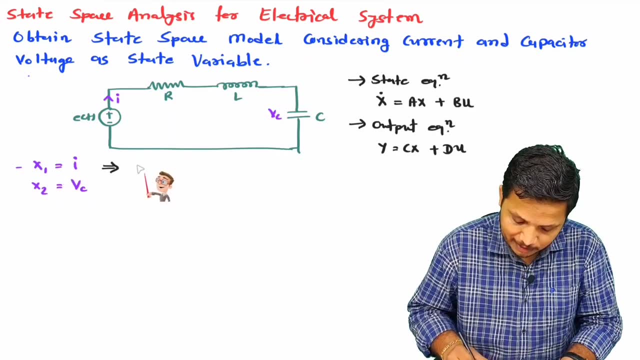 of input signal right, And here, if you observe, input is ET right. So if you differentiate X1. Then you will be having X1 bar and X2 bar in terms of input signal right, And here, if you observe, input is ET right. So if you differentiate X1, then you will be having X1 bar and X2 bar. 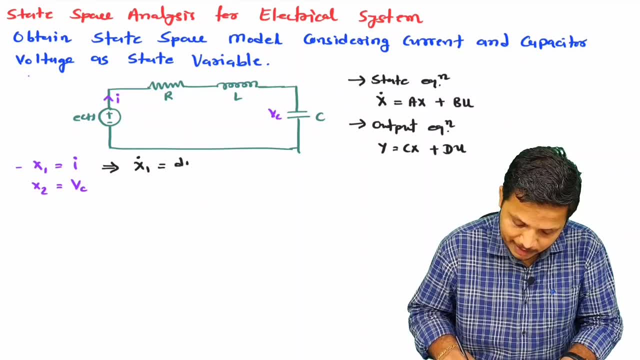 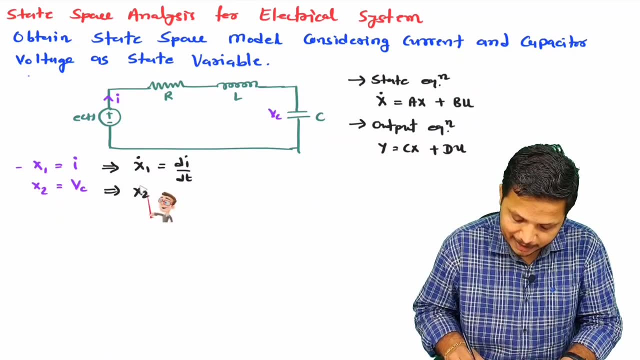 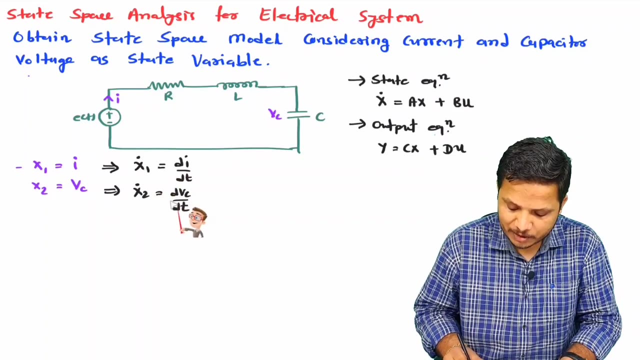 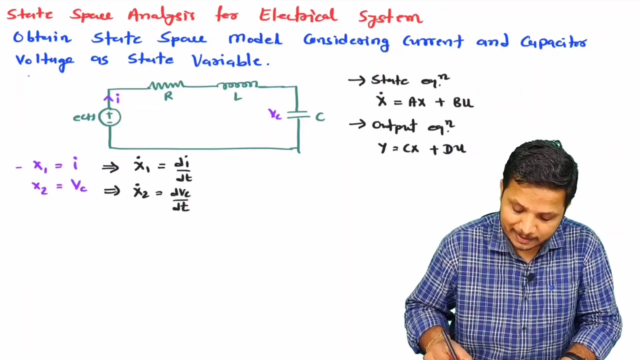 and this is what DI by DT, that one can say, and if you differentiate X2, so that is X2 bar and that is DVC by DT, right? So this is what we will be using in future equations. So just take care of this. Now let us consider first this loop and based on this loop, we will be. 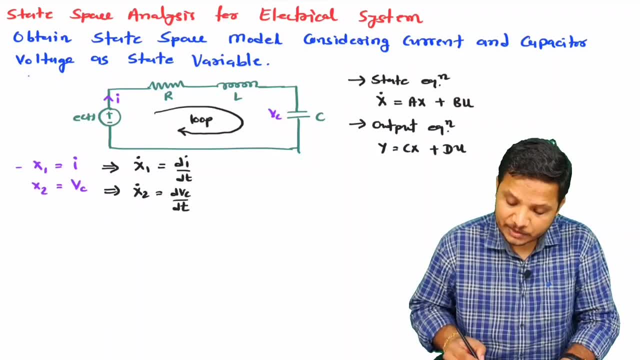 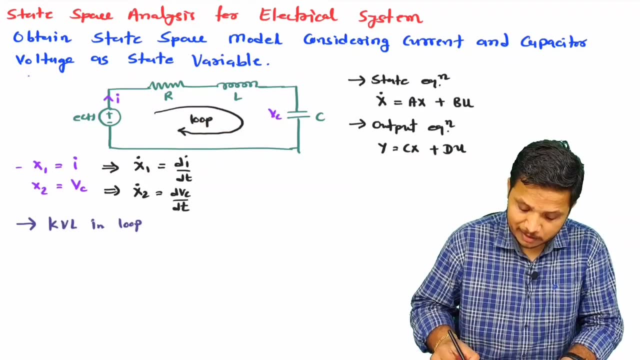 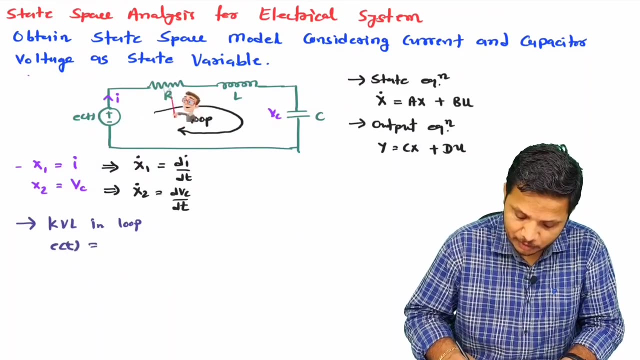 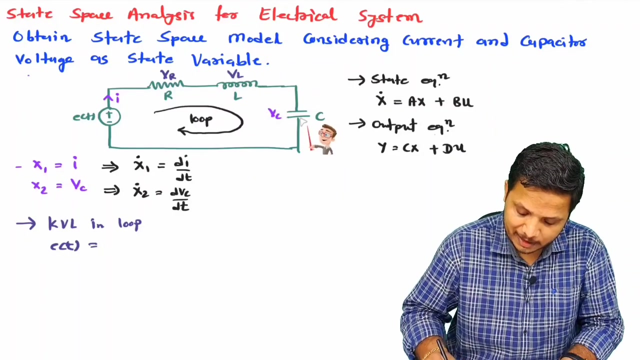 identifying state equations in differential form first. So if we apply KVL here, then E of T, that is, equals to voltage across resistance, let us say it is VR. voltage across inductance, let us say that is VL. and voltage across capacitance, let us say that is VC, So that will be VR. 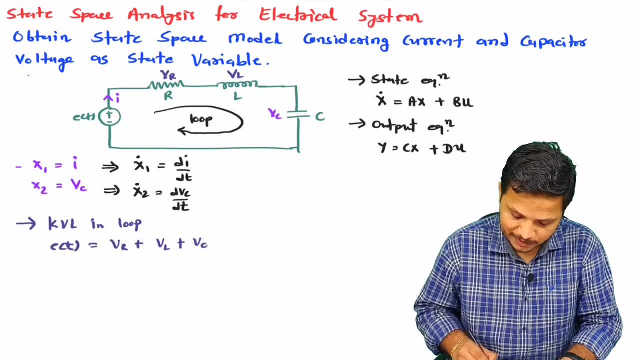 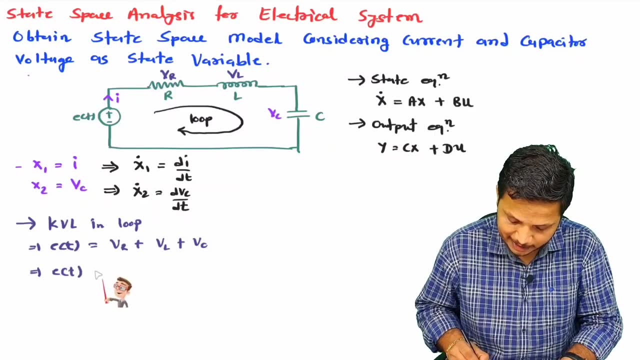 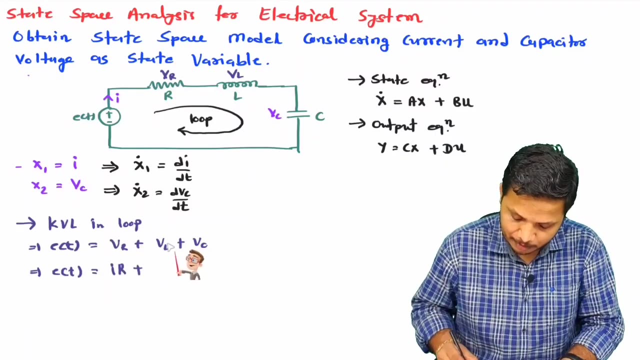 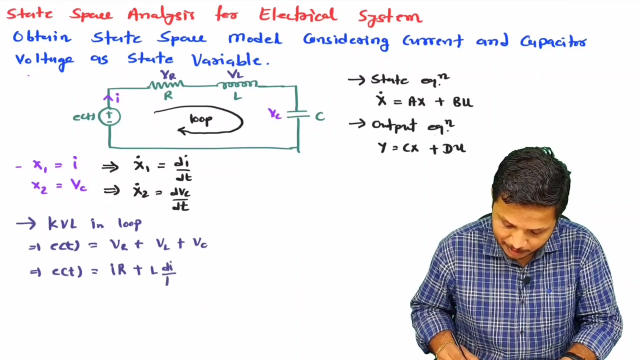 Plus VL plus VC. Now this EMF E of T. let us further simplify this. So VR is how much that is current I into resistance R plus what is VL? VL is L into DI by DT, inductance voltage, that is LDI by DT. 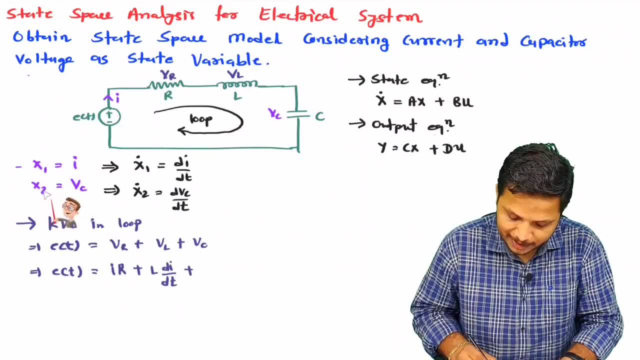 And VC is current I into resistance R plus what is VL? VL is L into DI by DT inductance voltage, that is, LDI by DT And VC. that we have already as variable. So I am considering that as VC only. Now you. 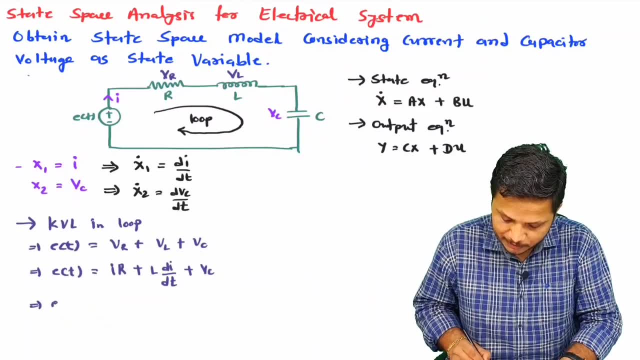 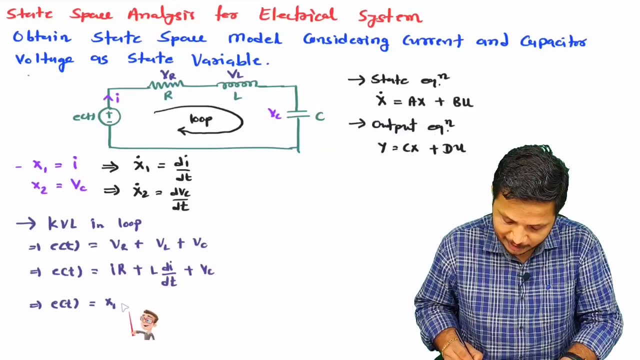 see E of T. that is my input, So I am just considering that as E of T. But you see, I, that is X1.. So I am writing I as X1 into R plus LDI by DT. Now, you see, DI by DT is. 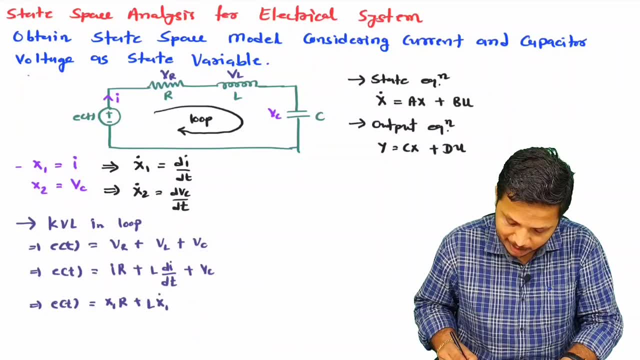 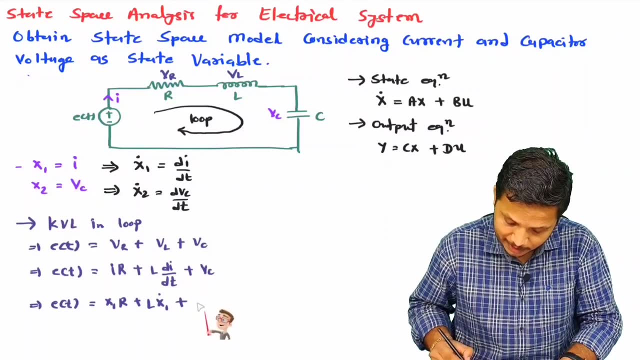 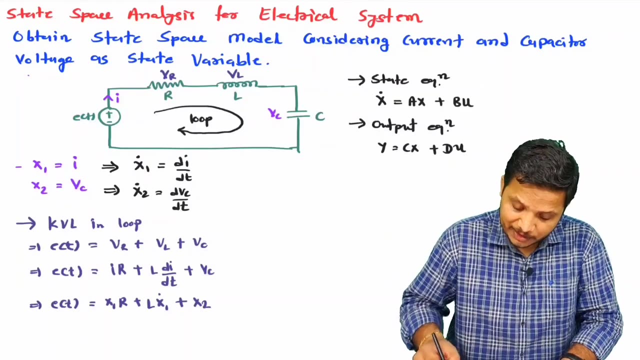 X1 bar, So LX1 bar that I need to write Uh, and then you have adversarial E as M1 by trail E by 1 plus VCE. Right, that is X2, that you see some red writing that as X2.. So I can have one differential. 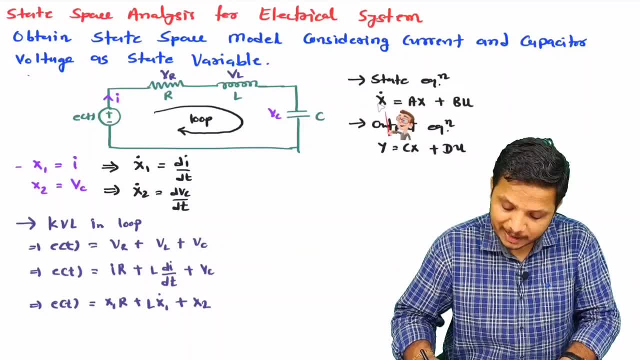 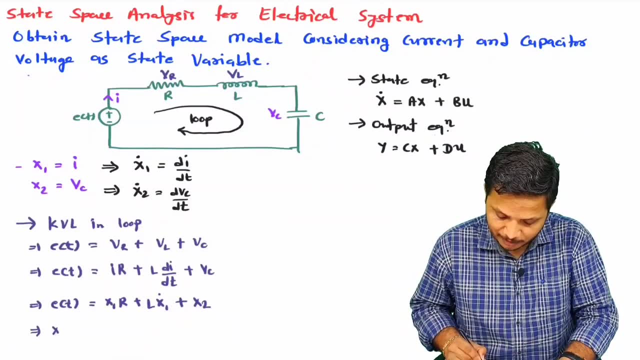 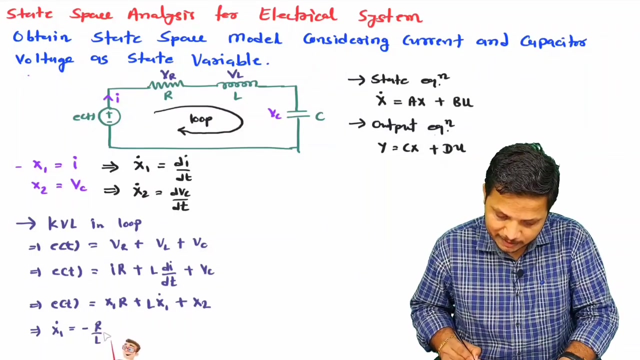 EQ. Right, you see X1 bar form that I need to have. So he had x1 bar That I am having, So I'm just making that as a main term. So x1 bar that is equals to- now you see this, this term that will go on other side. so minus r divided by l, as l will get divided over this side. 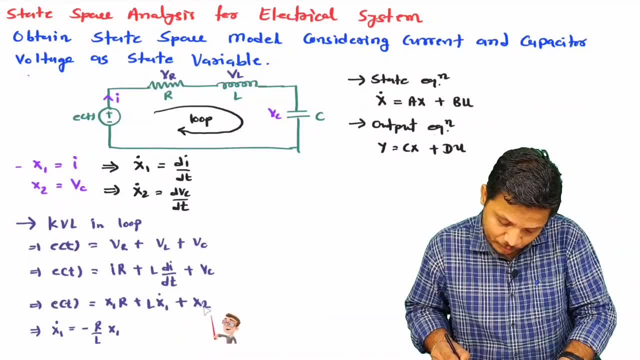 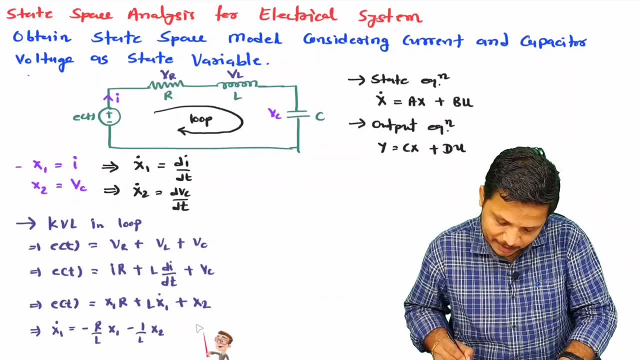 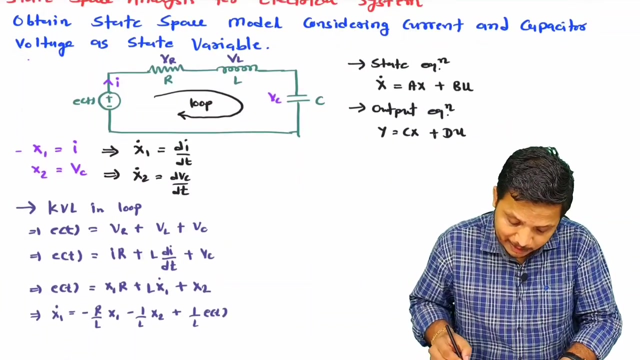 into x1, then x2 that will go over other side, so that will be minus and 1 by l- x2 that will be there with us- plus 1 by l into e of t. that is how one differential equation that is there with us right now. let us try to identify second differential equation, that is what, based on x2. 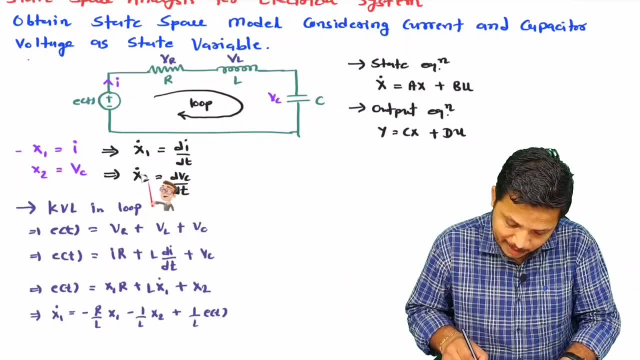 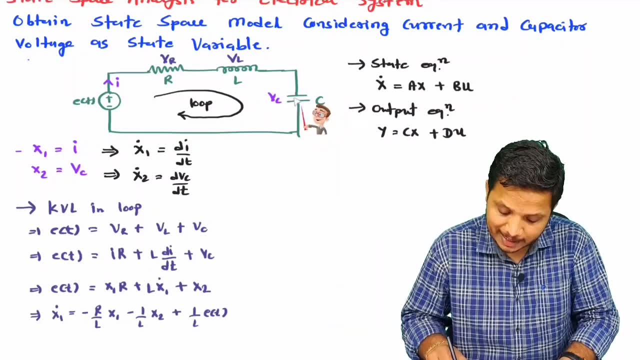 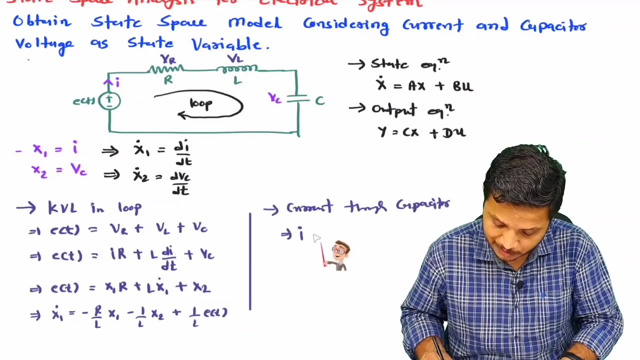 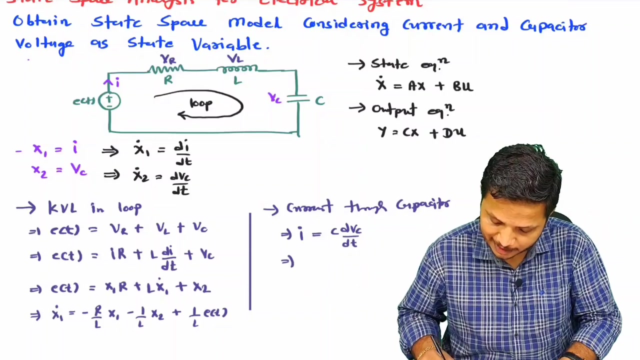 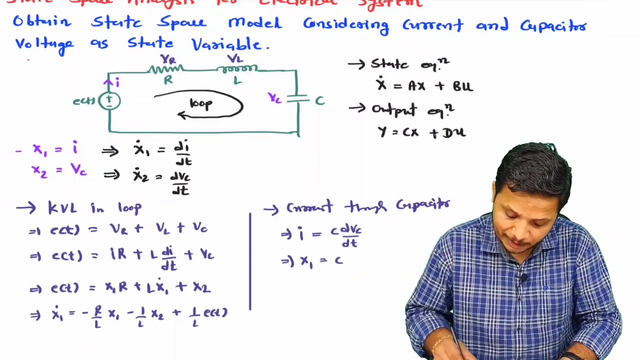 bar and if you want to have this second equation in terms of x2 bar, then we can directly consider voltage across capacitance, right, and that is having a relation of current. so we can say: current passing through capacitor is i, is equals to c into dvc by dt, here i is x1, that one can say that is equals to c into vc, that is x2. 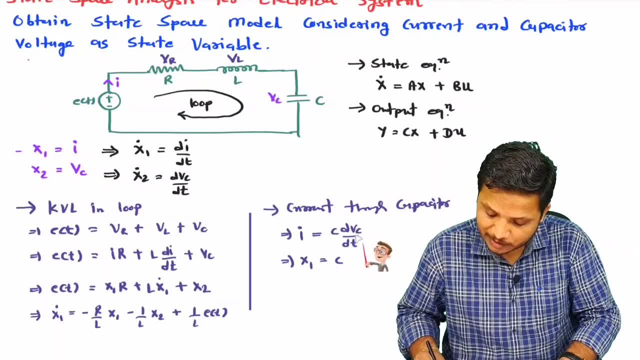 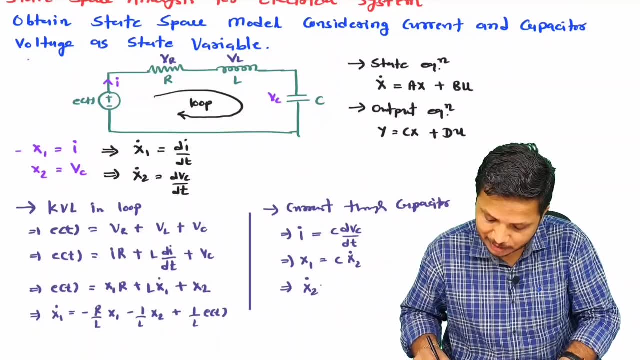 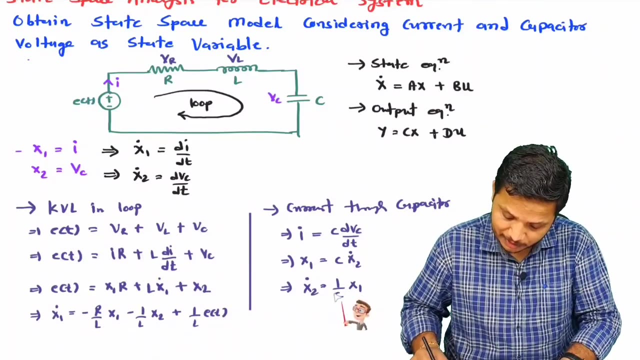 you see. so this is x2 differentiation means we can say x2 bar. so here we will be having x2 bar equation that is 1 by c into x1. so now we have these two equation and that we can use it to form first state equation. 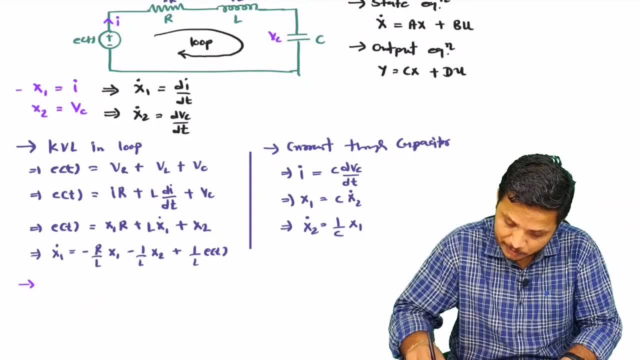 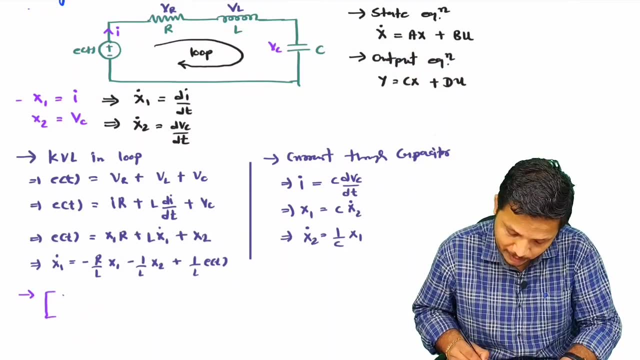 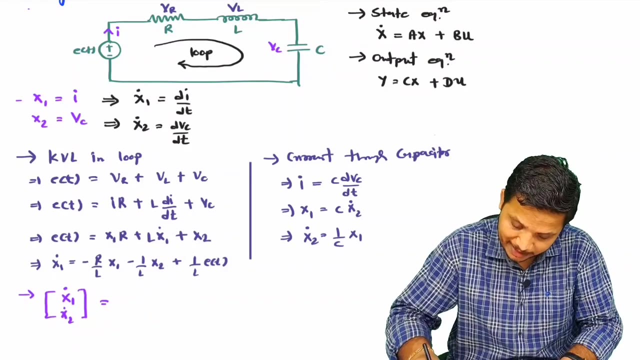 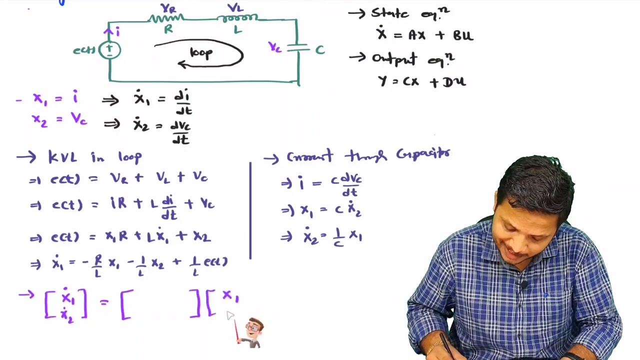 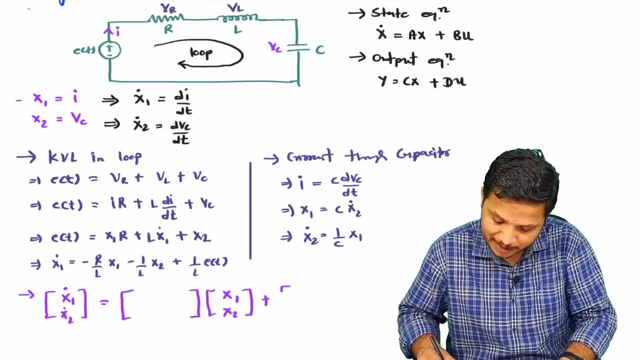 let us consider that. so first state equation, that is x bar. right, here we have x1 and x2. so i need two right: x1 bar and x2 bar. that is equals to matrix a. that i'll write over here into x. so here we have two variables, x1 and x2, plus bu, where b that will be our another matrix. 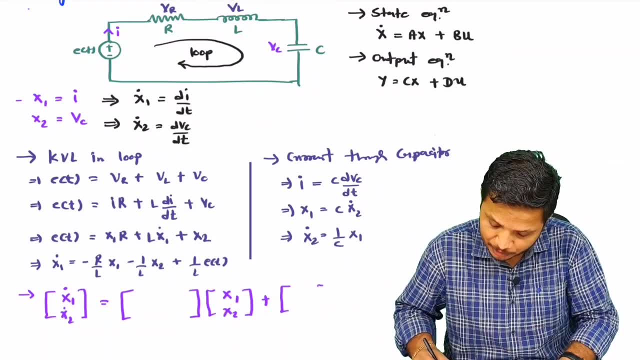 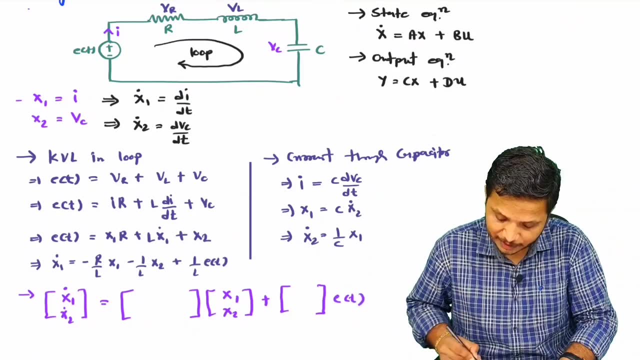 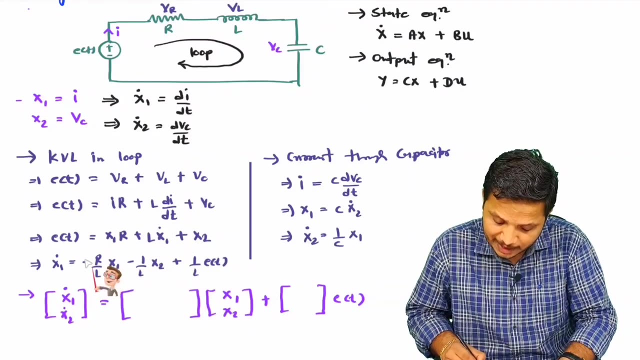 into u. that is our input. and here we have input that is e of t. so i'm writing: my input is e of t. now you see from first equation, here x1 is having coefficient, that is minus r by l. so here minus r by l, that will be having. 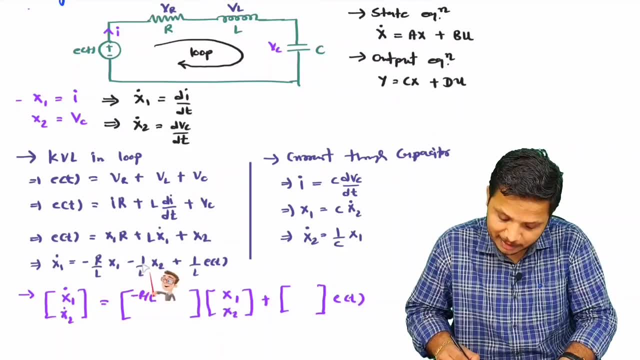 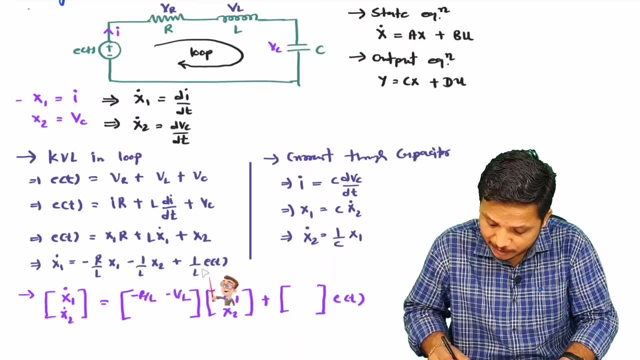 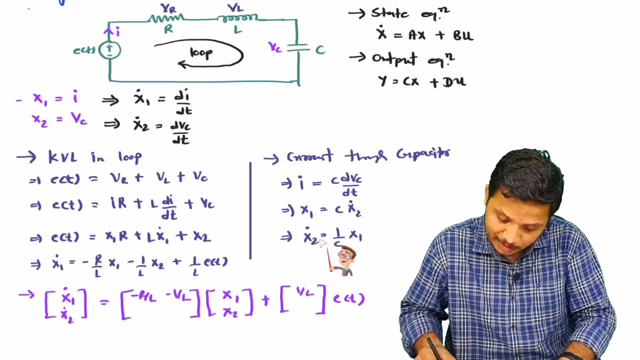 and x2 is having coefficient over here that is minus 1 by l, so minus 1 by l that i need to write. and input is having coefficient- 1 by l, so 1 by l that i need to write. and if you see x2 bar, so x2 bar. 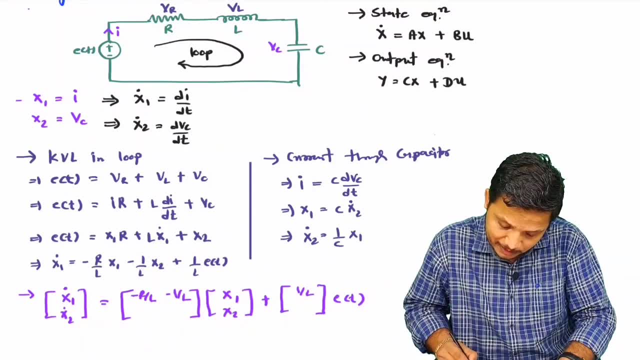 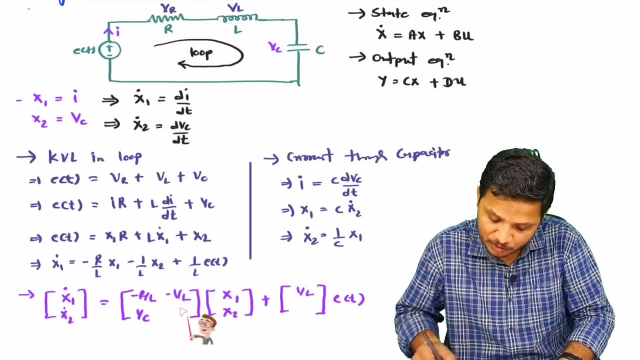 that is having x1 coefficient, that is 1 by c. so i'm writing 1 by c and we don't have any other thing. we don't have x2 coefficient, so this is 0, and we don't have input coefficient, so this is even. 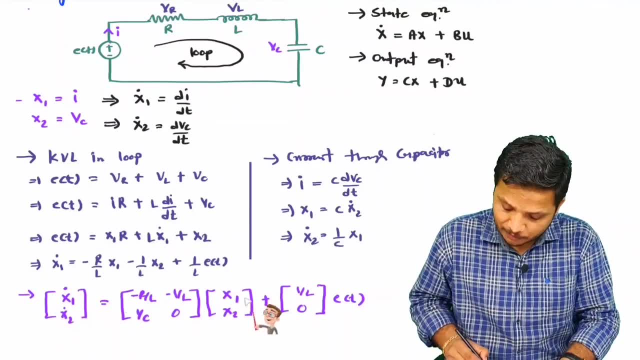 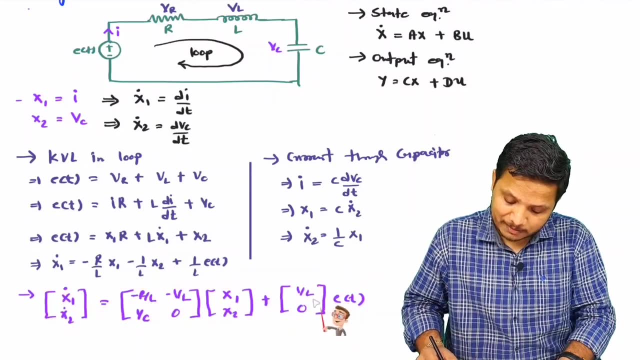 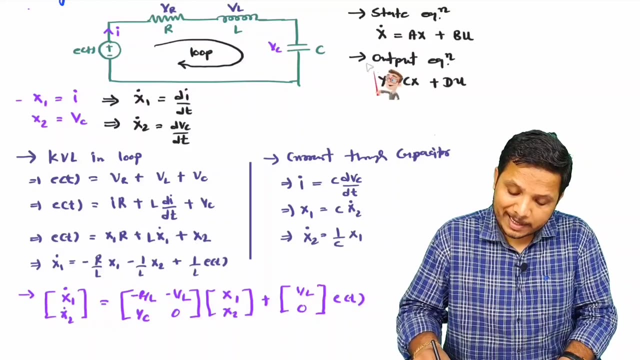 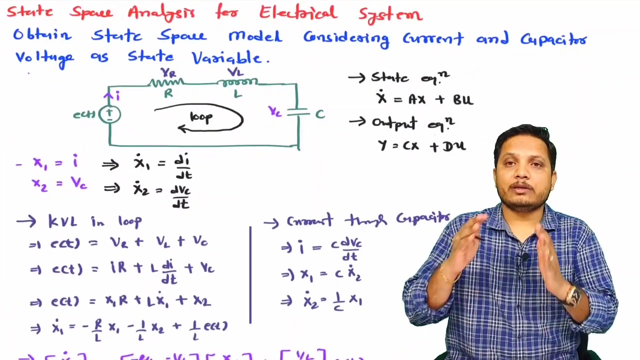 0. so this is how we have state equation over here, where this is matrix a, which is system matrix, and this is matrix b, that is our input matrix. right now, we are delivered to identify output equation for this. now, whenever you have this type of question- one thing that you need to keep in. 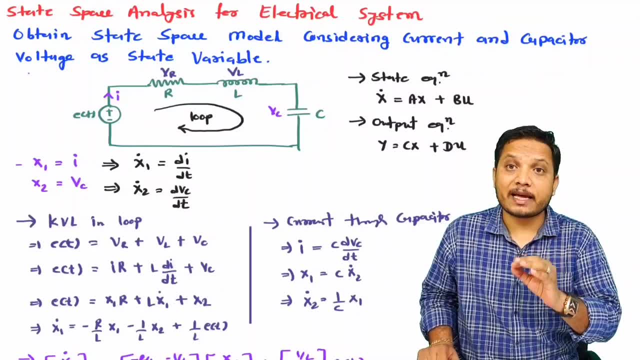 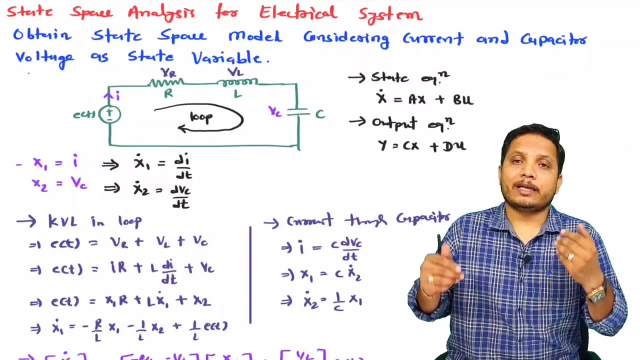 your mind. see, in output matrix there can be one. in your input matrix there can be only one. matrix be any number of outputs, right? it is not like there are two outputs only. you can have two outputs. you can have one output, you can have three output. it is your wish how many outputs. 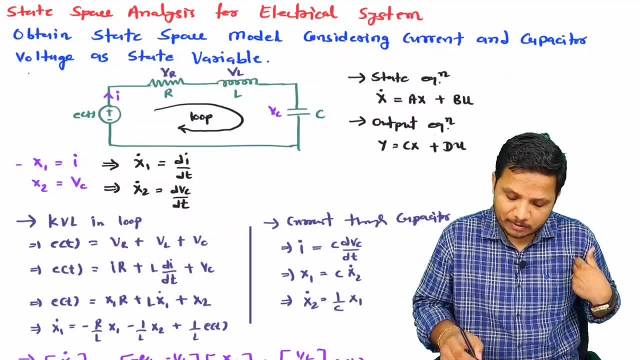 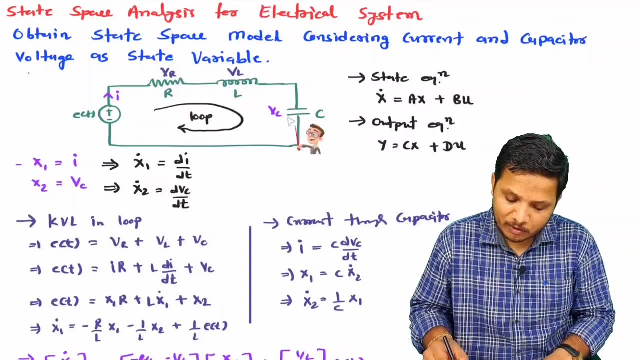 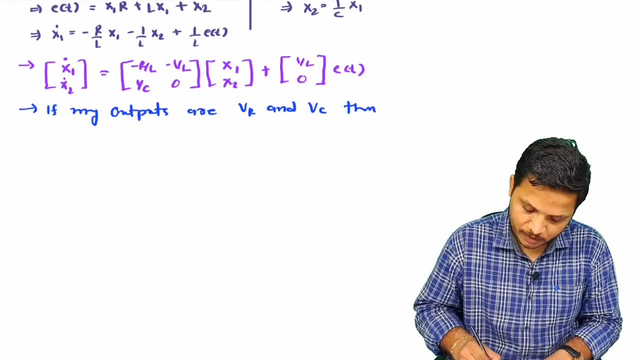 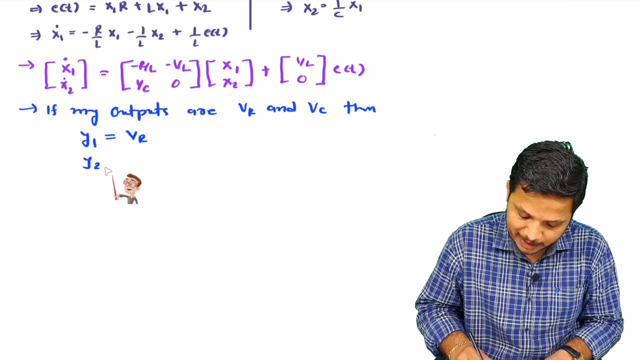 that you want to take right? So here, if you observe the circuit where we can have many outputs, but I am just going to consider output across resistance and output across capacitance, right? So if I consider that, then my one output that is, let us say, that is y1, so that is vr, and my second output, let us 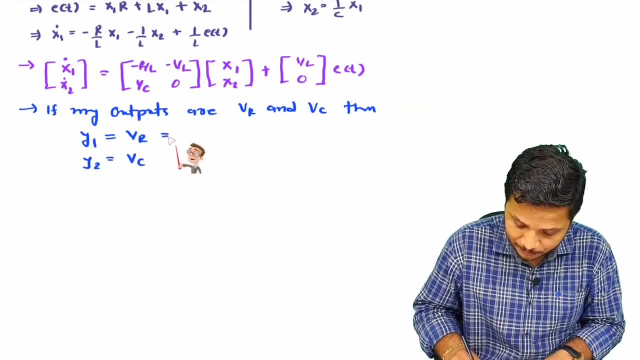 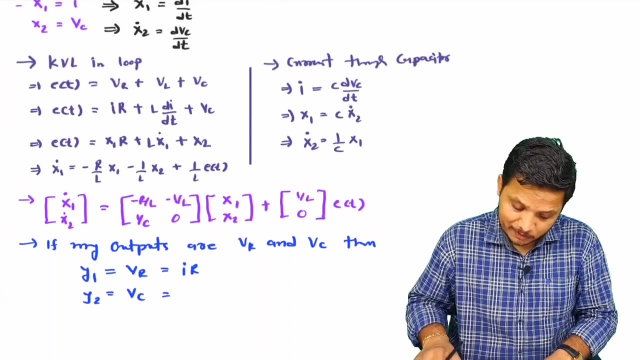 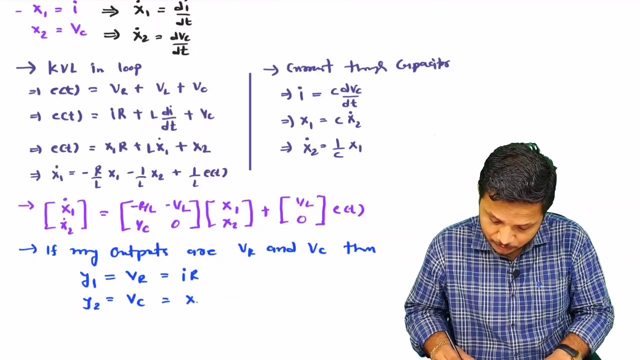 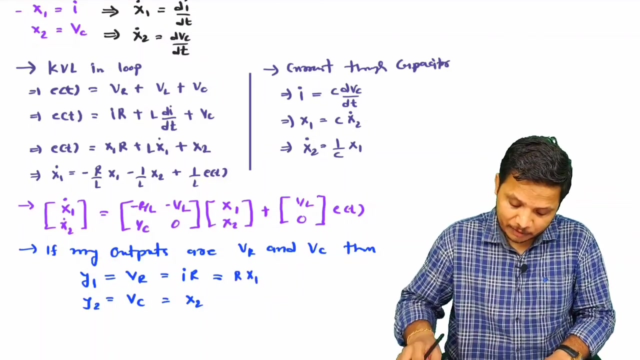 say that is y2, so that is vc. now you see, vr, that is i into r and vc, right, so that we already have see: vc is x2. so I am placing vc is x2 and i into r where i is x1.. So r- x1 that we need to say. 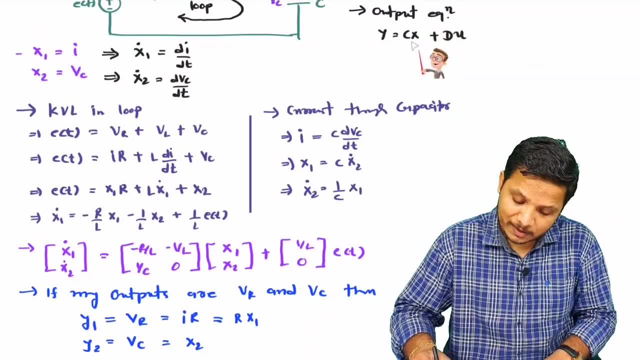 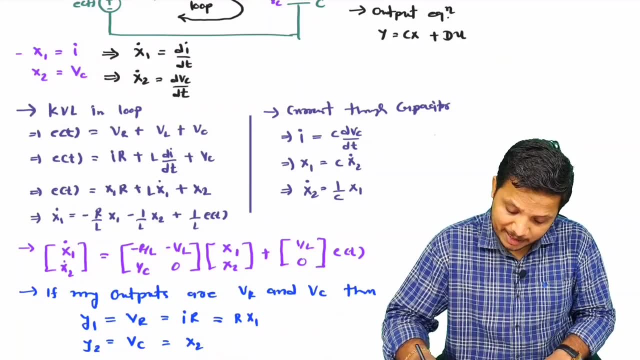 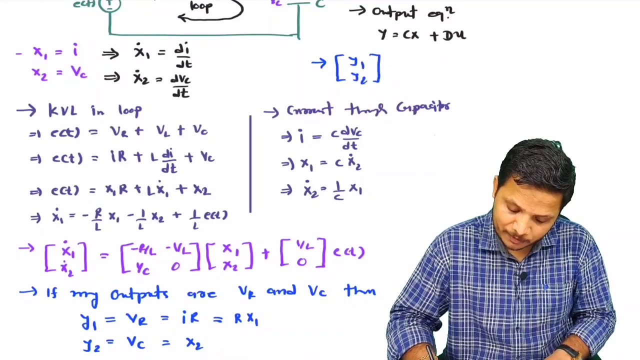 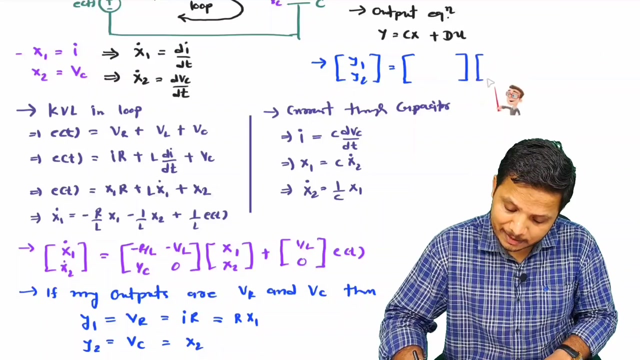 Now, if you see, our output equation, that is y, is equals to cx plus du right. So based on this we can form this. now see, I am making that equation here itself. So here my output is y1 and y2, that is, equals to matrix C that I will write later into x. 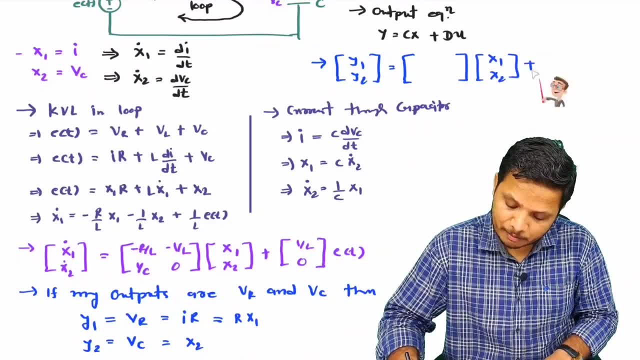 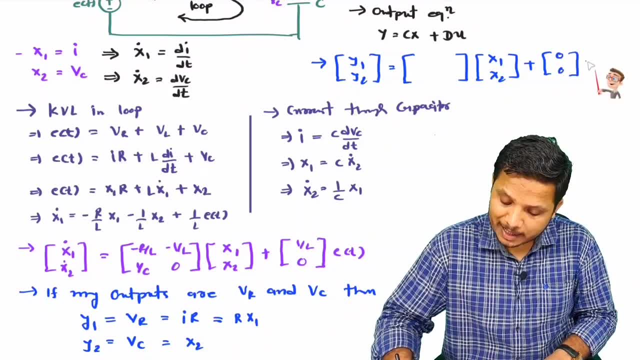 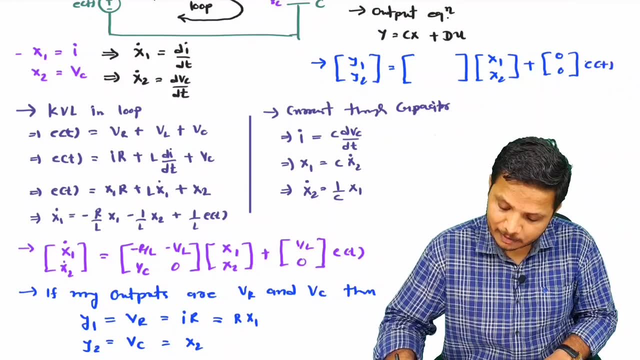 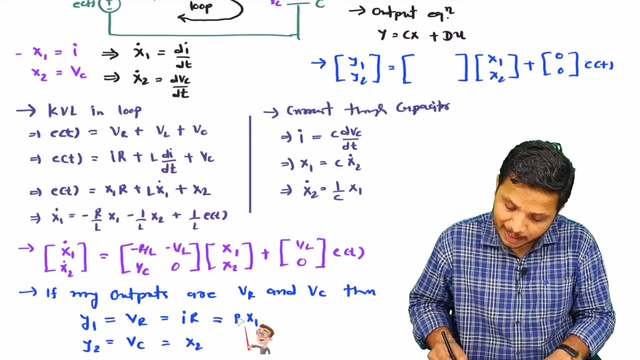 here 0, 0 that I need to write an input that is e of t, which we have. input is e of t. Now, if you observe y1, so that is having r, x1, so x1 is having component r, so here I am writing r. we don't have x1. 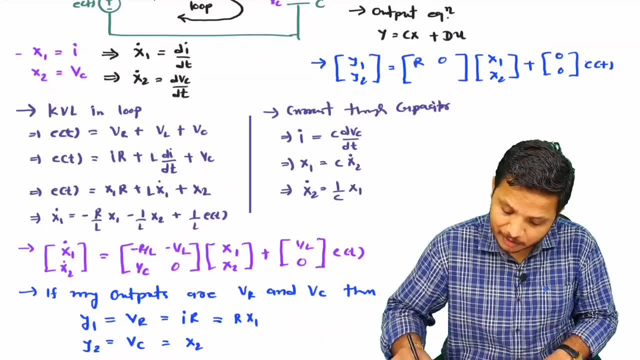 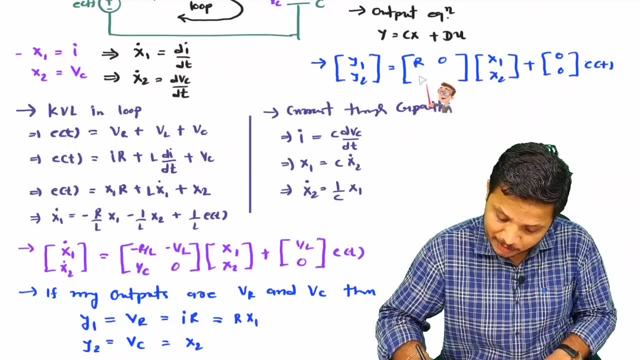 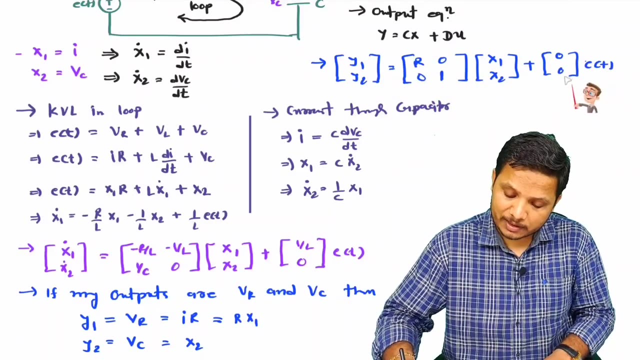 So x2 component. so here x2 component will be 0 and if you observe y2 equation, so that is having vc, which is x2, so x2 is having 1 component which is over here, and x1 component is 0.. So this is our output equation for this modeling. if you have 3 output, then y1, y2, y3 and here.